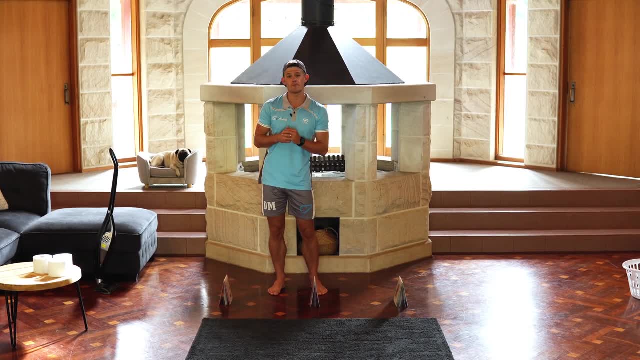 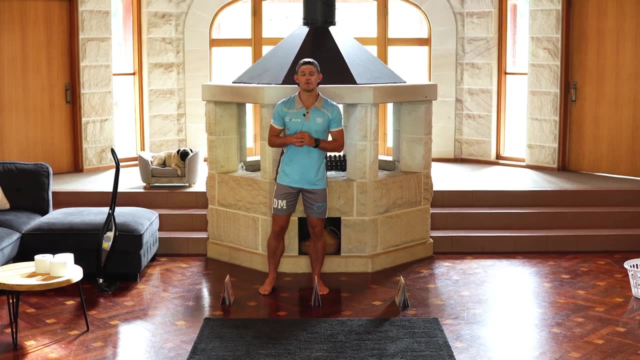 Now I'm going to show you a couple of stations. When you do your stations at your home, you're going to do them for 30 seconds and then you're going to have a 15 second rest in between each one before moving on to the next one. 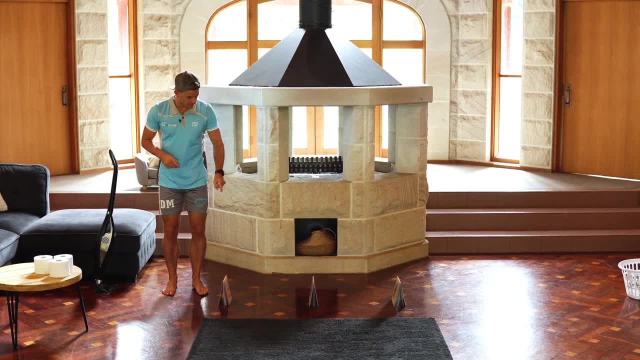 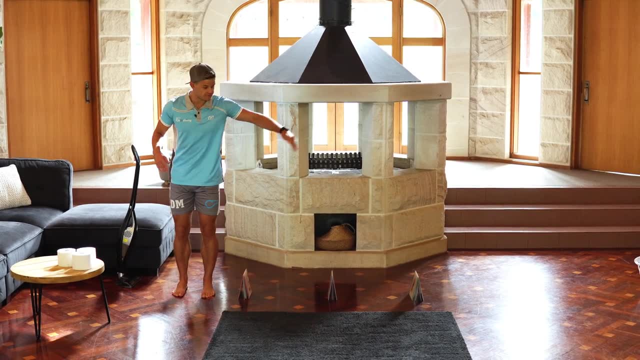 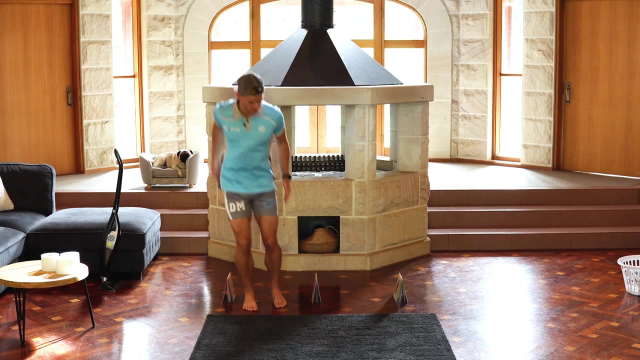 So let's get started. The first station: I've got three books and I've spaced them about half a metre apart. You're going to do two footed jumps over them left and right. Here we go, Keeping feet together, jumping sideways two feet up and over the books. Try not to knock them down. 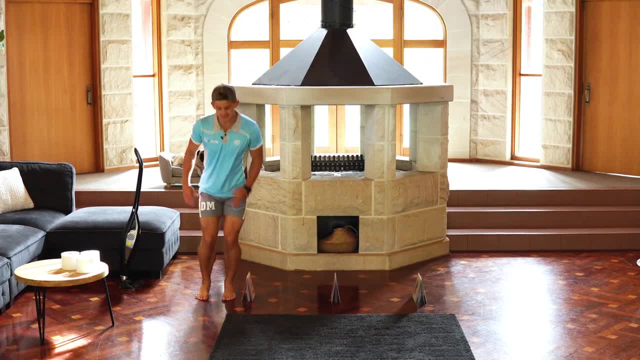 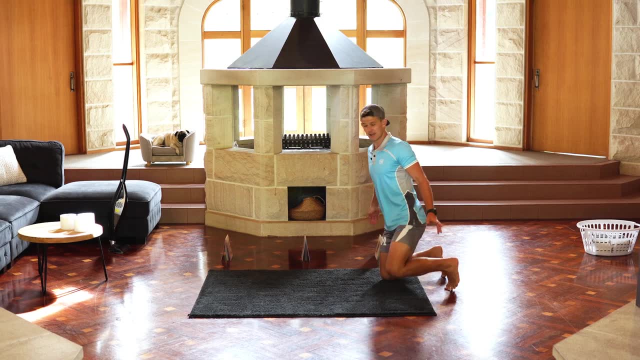 Remember, each station you do for 30 seconds, until time is up. The next one we're going to do is a plank. A soft spot on your carpet. You can maybe put a towel down. We're going to do a plank, So we're going to lay nice and straight on the ground. 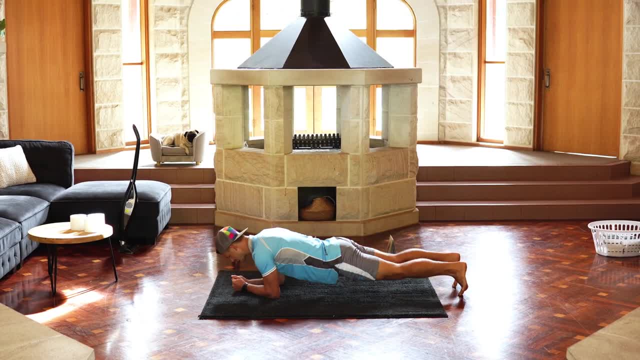 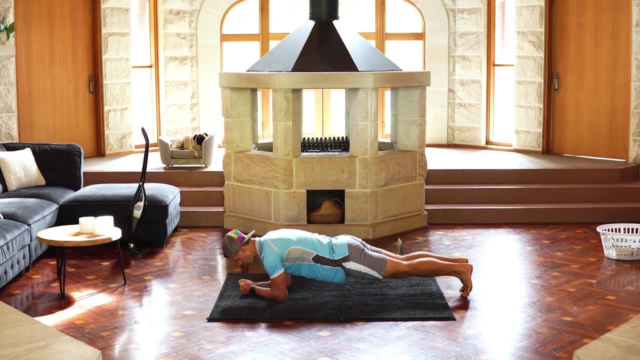 This is a plank, That's not a plank And that's not a plank. You can see, my back is nice and straight and my bum is nice and straight as well. Strong and straight. Hold that straight, Balancing on your elbows, for 30 seconds and then you're done. 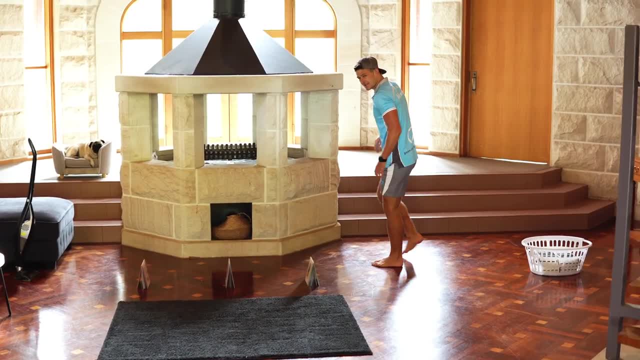 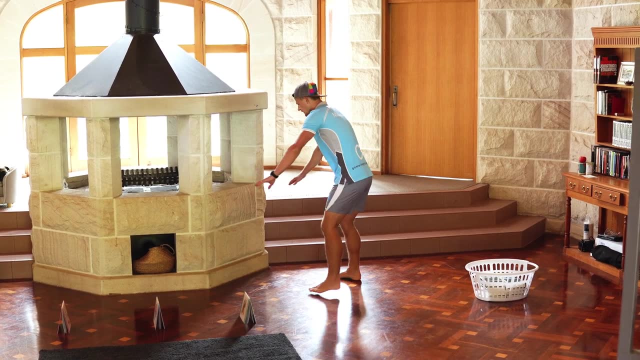 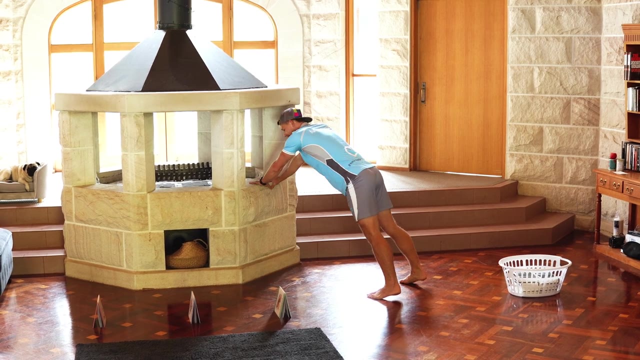 Okay, next one: You need to find yourself a ledge, Something that's strong, about chest height or sturdier. We're going to do a stomach height and we're going to do one-handed push-ups, okay. So start off with two hands. You take one hand off and you're just going to push down and up again. 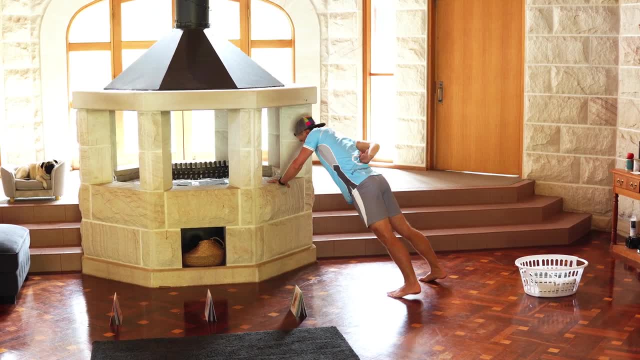 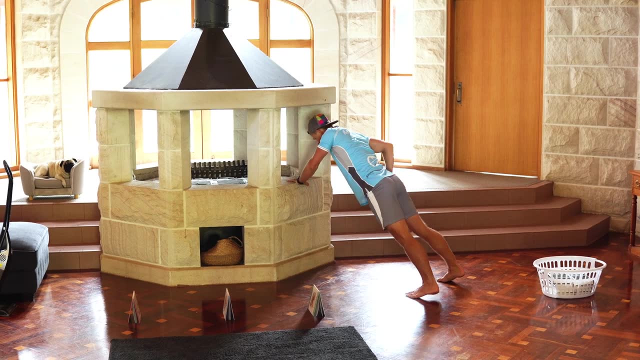 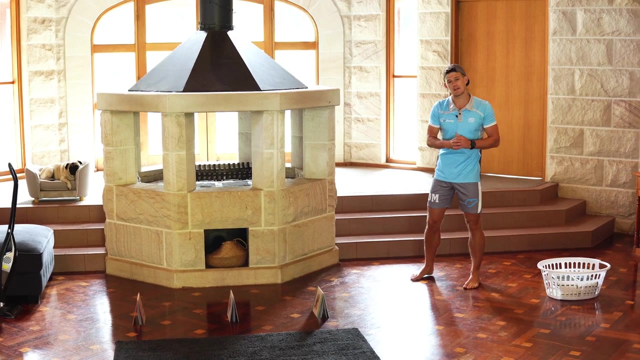 And then switch hands. okay, It's not easy. Switch hands each time. You're going to do as many as you can in 30 seconds. Okay, we'll do one more here. There we go, Okay, if you have some steps in your house. 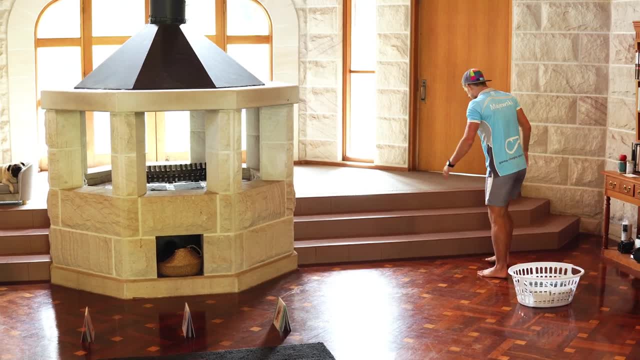 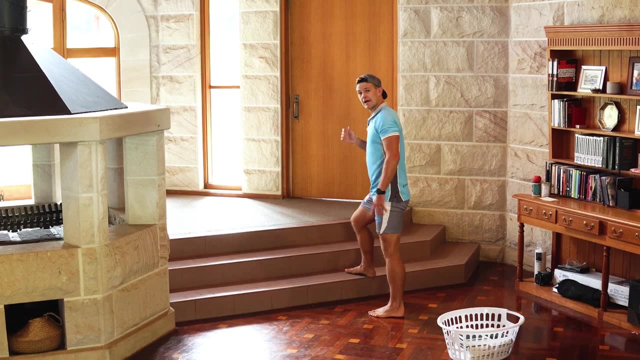 Here's another one. Here's another exercise we can do. So you're going to step up with one foot, You're going to bring your opposite knee up and touch your elbow to that opposite knee and step back down. You're then going to switch feet. 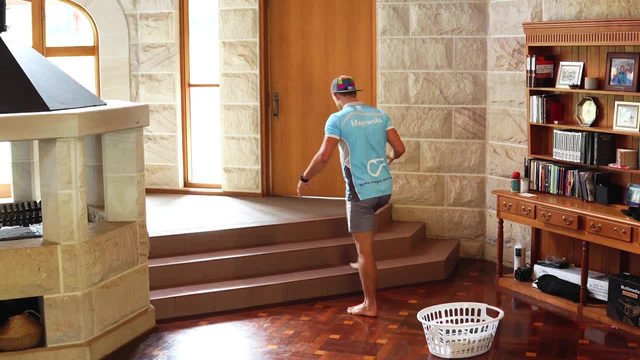 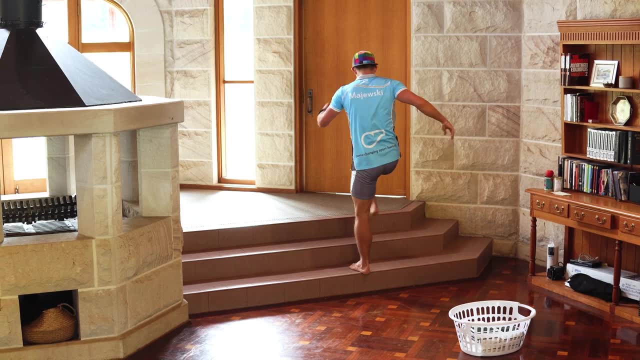 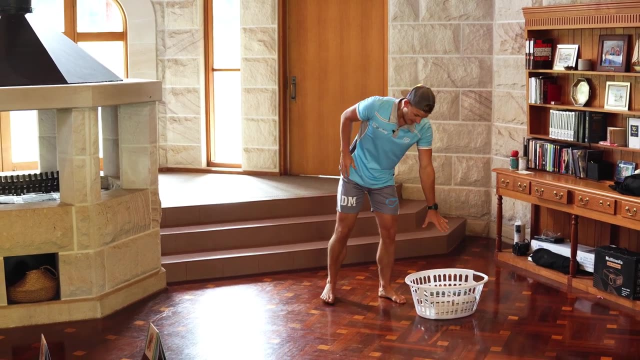 Okay, so step up Opposite elbow to opposite knee. Make sure you're safe. Don't trip on the stairs. Awesome, You do that for 30 seconds. Okay, if you have a laundry basket, You're going to get one and you're going to fill it with a couple of heavy things. 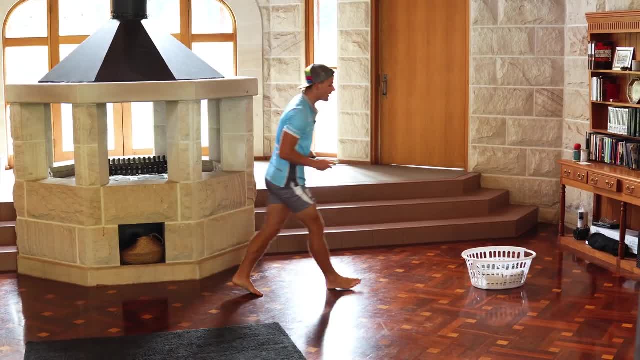 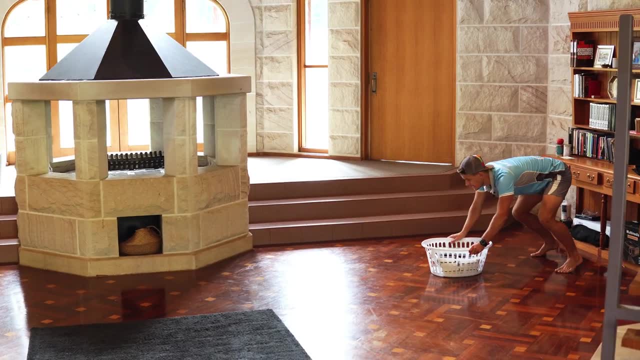 I've put some books in there. I might put these ones in as well to make it a little harder, And you need a nice space in your house that you can push it up and down. So you're going to get down low back straight. 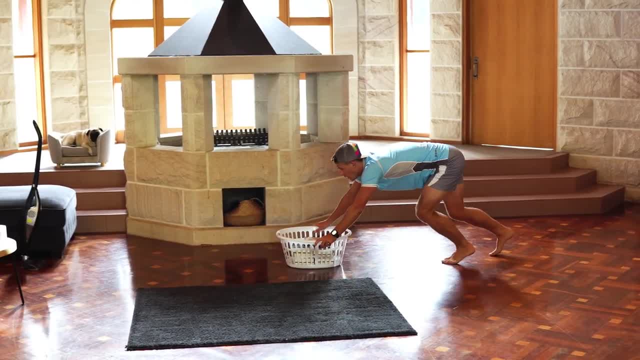 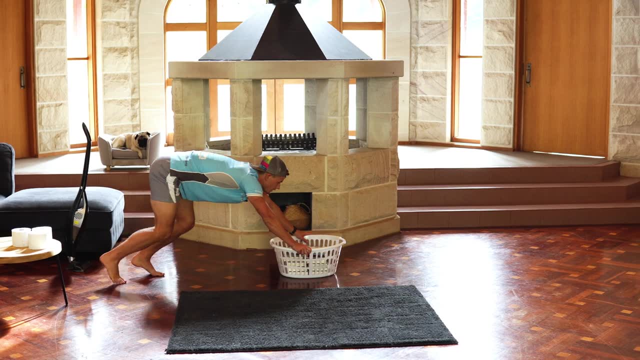 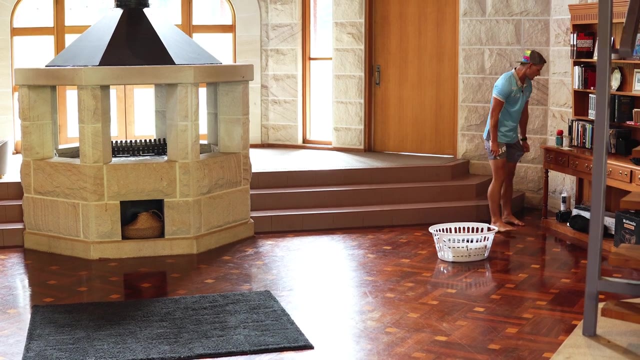 And with two hands you're just going to push, sliding it across the floor backwards and forwards. Okay, remember staying low, Using your legs to really drive that. Okay, next one we're going to do On some steps. you're going to squat down the steps. 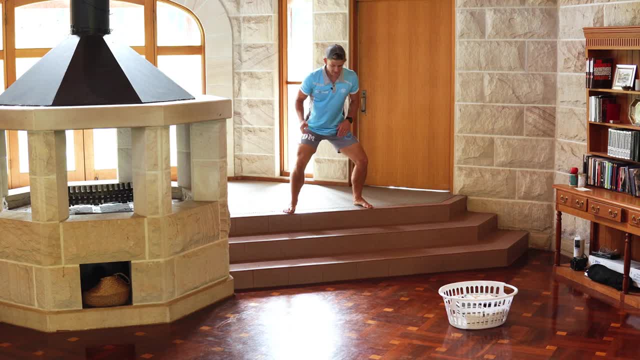 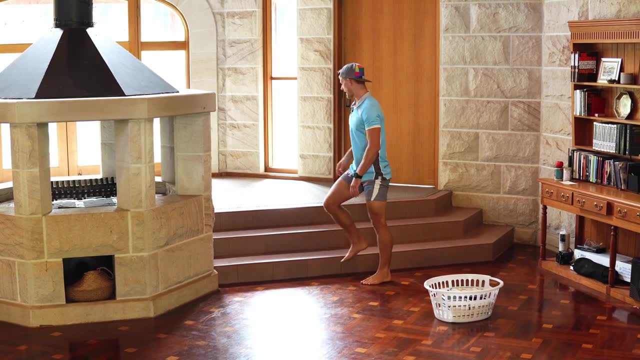 So now start at about the third or fourth step. You're going to keep your legs bent And you're just going to jump down to the next one keeping your back straight. Okay, walk back up. Be nice and careful with this one. 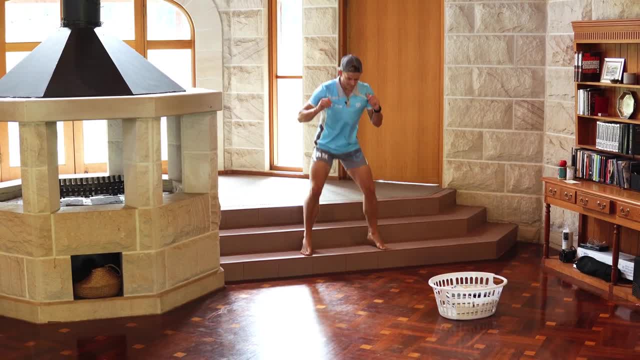 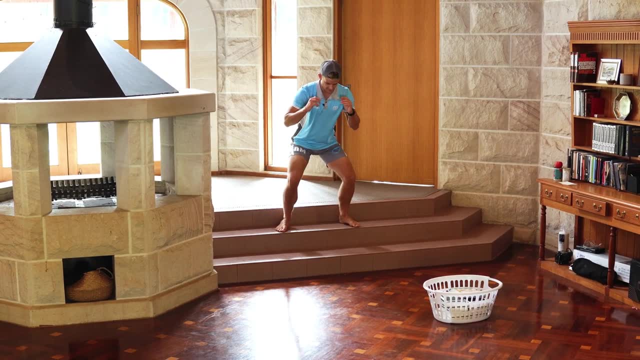 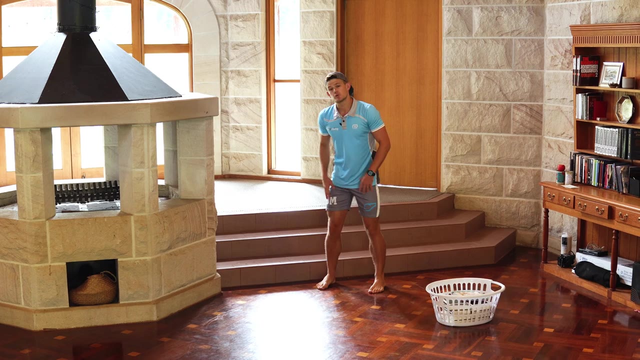 You don't want anyone falling over. Remember, each station is for 30 seconds. One more. here I'm going to do Awesome. Okay, Something else you can do on the steps: You can do tricep dips. So here you're going to get to the first step. 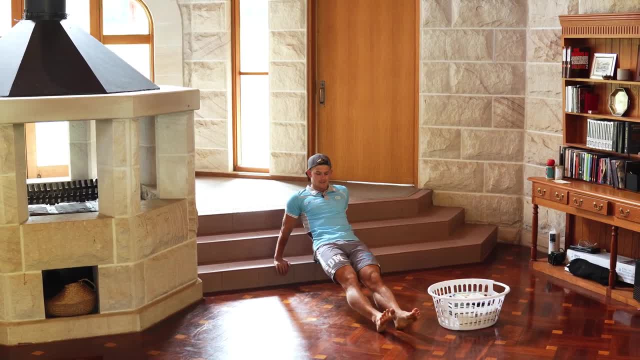 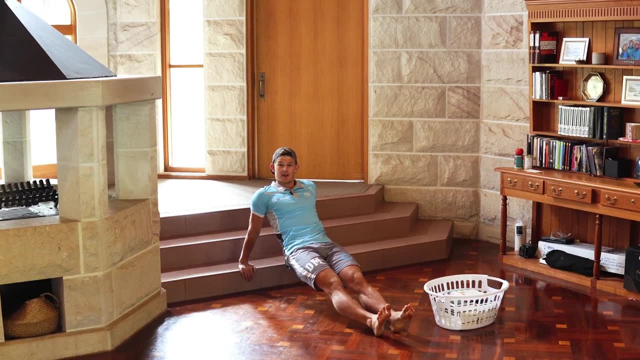 You've got to put your body up, nice and strong and straight, And you can see my body is straight And now we're just going to dip down. Gently touch my bottom to the ground And come back up. So dip down. 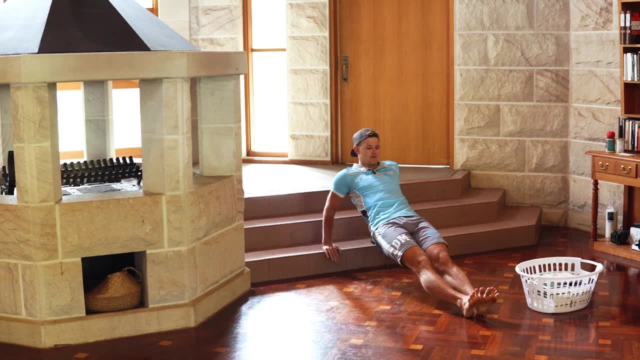 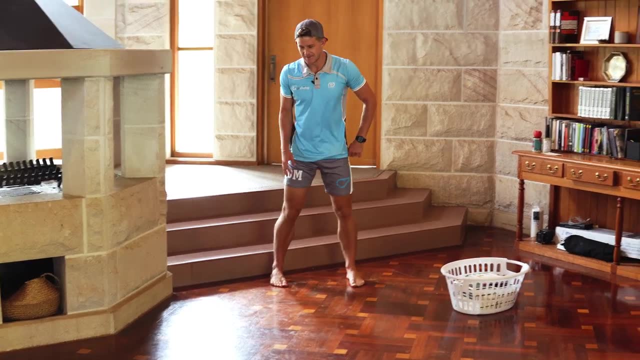 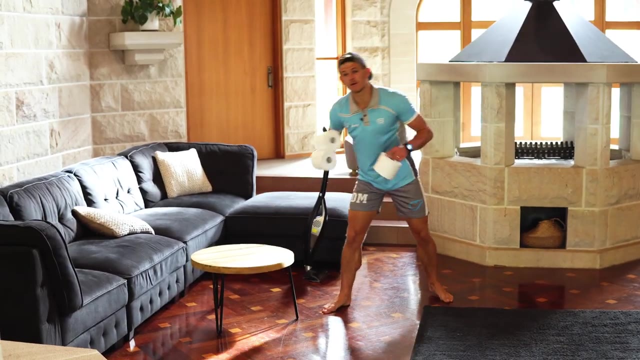 And up With both hands, nice and carefully controlled, Working on your triceps. That's the back of your arms, just here. Okay, next one: Toilet roll squats. You're going to get two or three toilet rolls And you're going to stack them just like that. 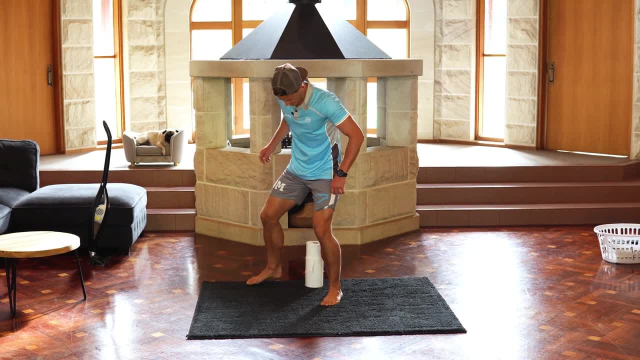 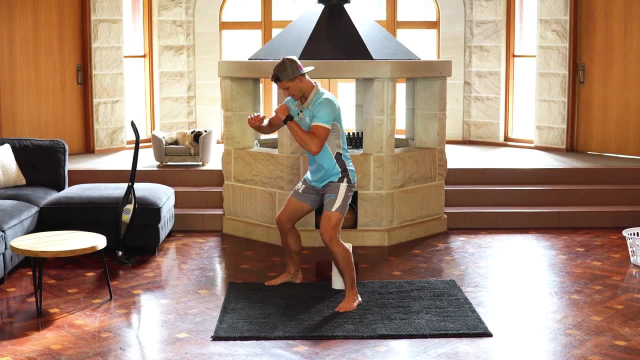 And what you're going to do. You're going to stand in front of them And you're just going to squat down until your bum touches them And then you jump up. Okay, and then we go again. Squat low, take your time. 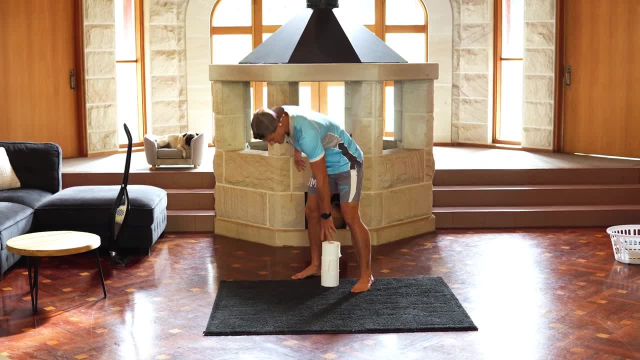 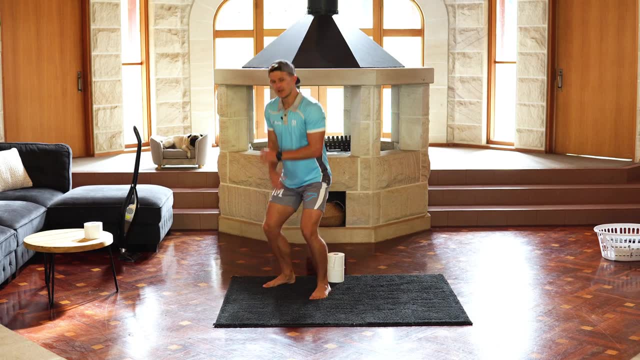 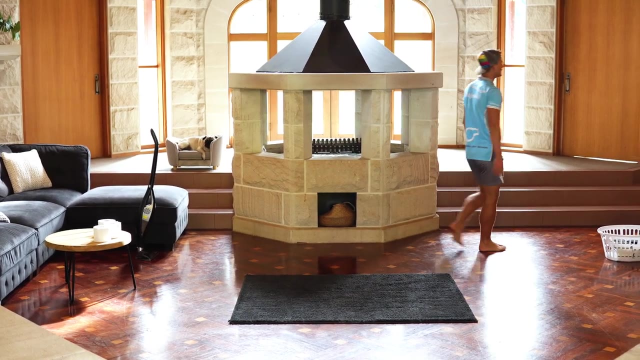 And jump up. We'll do one more here. If it's too easy, you can take one away. Makes it even harder, So once you touch, You can jump straight back up. Awesome, Okay, Another one I have for you. 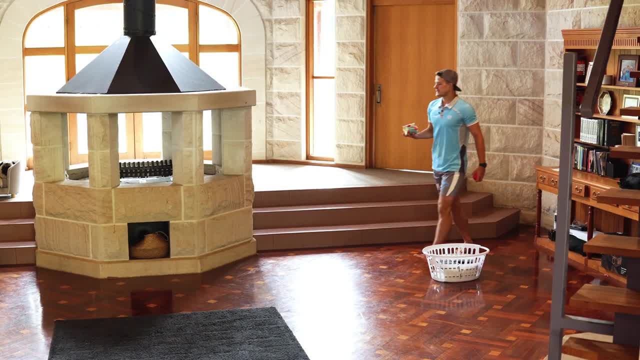 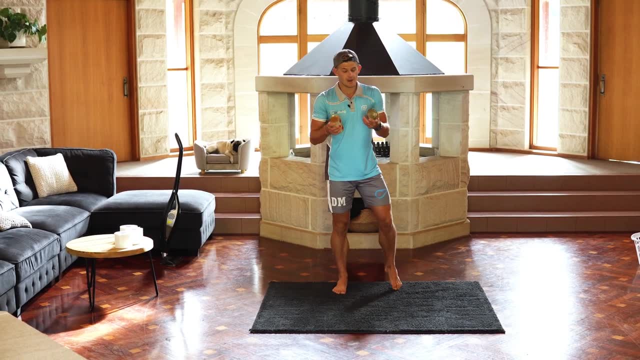 You need to go to the kitchen And you need to get yourself some cans of food. I personally like to use the tomatoes. If you can get the vegetarian tomatoes, They're probably better. Okay, One hand, One can in each hand. 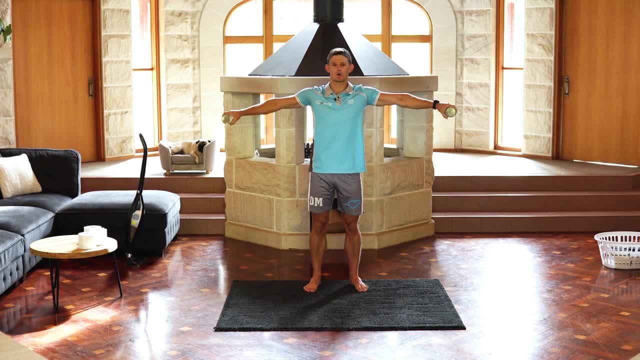 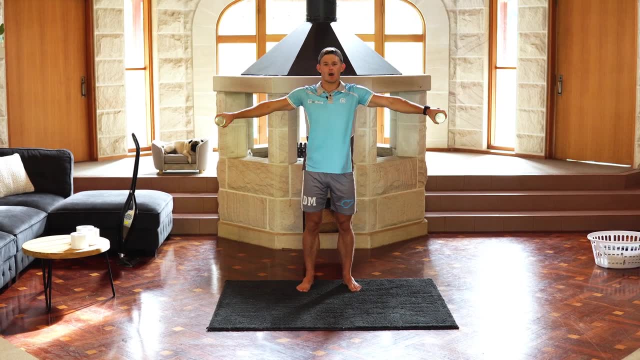 You're going to stand up nice and wide And you're just going to do big circles with them And you need to keep your arms straight. If you keep your arms bent, You're not really working on your shoulders. Okay, You need to keep your arms straight. 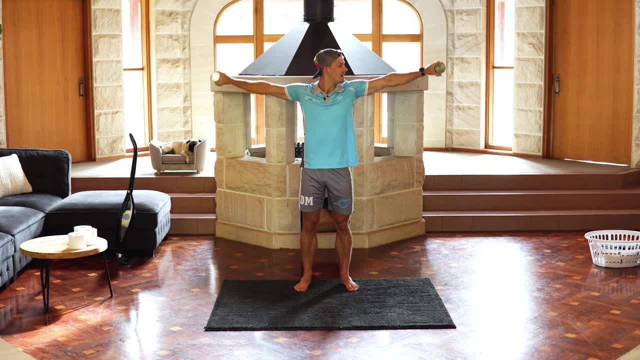 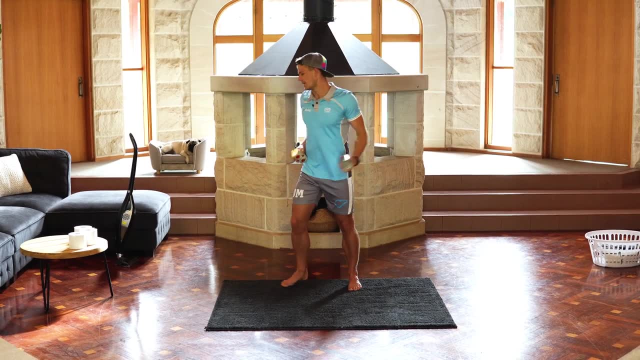 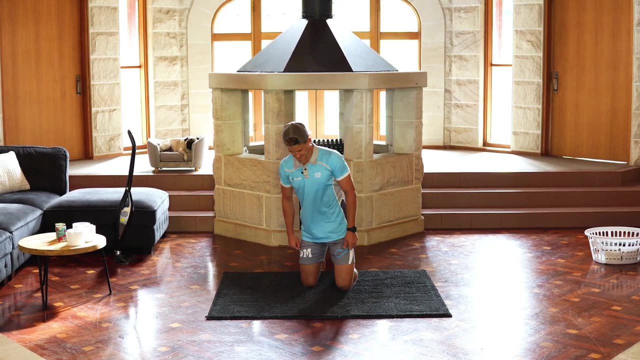 And you can go forward or backwards, Whatever you like. Okay, It's not easy to do that for 30 seconds, Awesome, Alright. Next one, Again On a nice soft spot. You're going to start off on your knees. 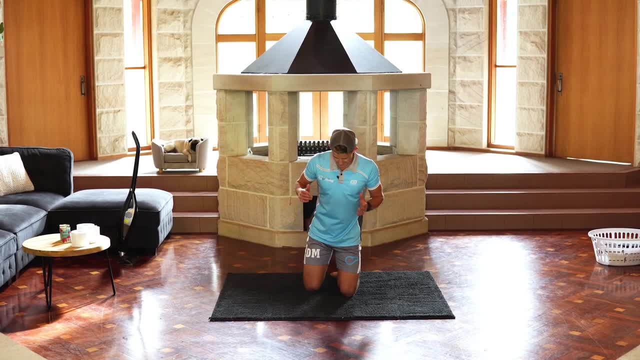 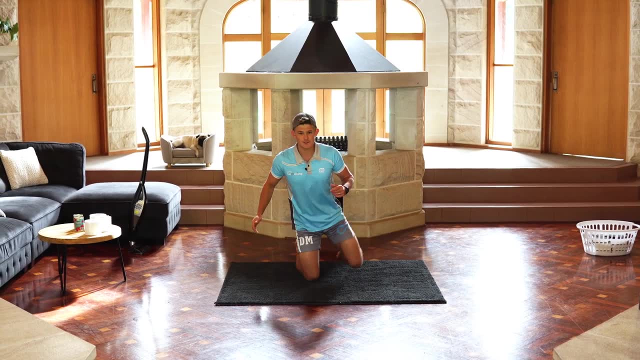 And you have to quickly jump up to your feet Without using your hands. So from here You've got to quickly jump up And then stand up, And then you come back down onto your knees Using your arms to swing, Jump up and stand up nice and safely. 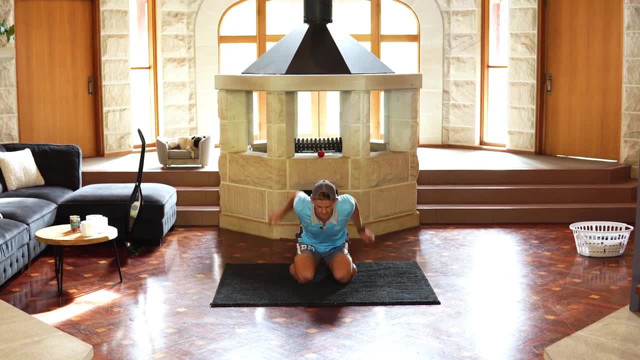 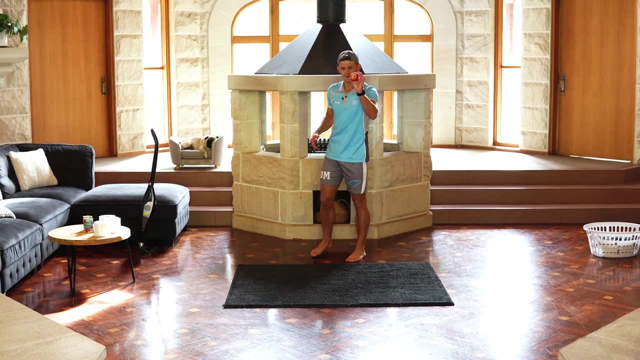 Let's go one more here. You've got to do it very quickly. There we go, Alright, Nearly there, Nearly there, Get an apple or a small ball, And we're going to do side planks. Okay, This time. 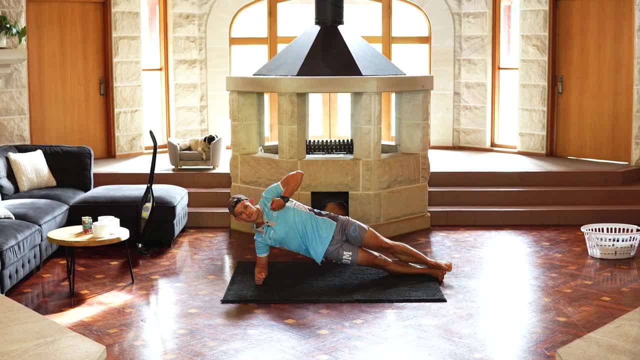 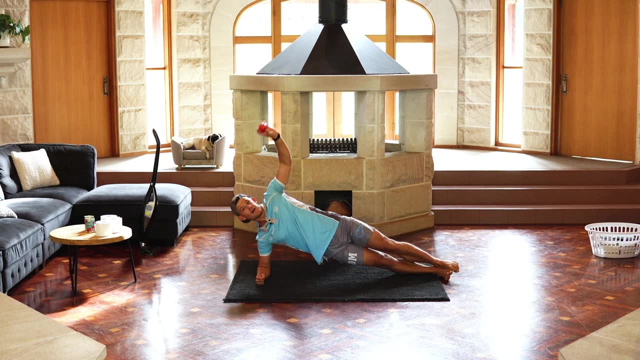 I'm leaning on my elbow, On my arm. You can see my body's nice and straight And it's off the ground. My hips aren't touching the ground. I'm nice and straight off the ground Holding my apple. I'm going to hold it nice and high. 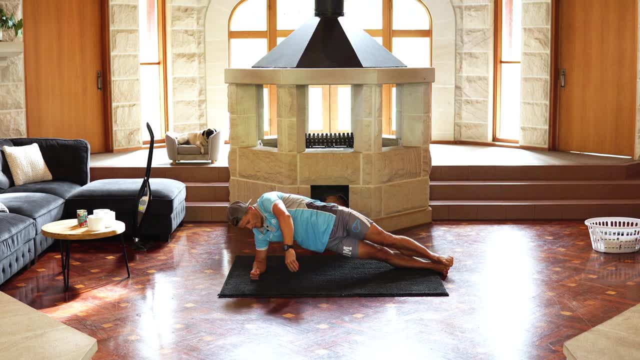 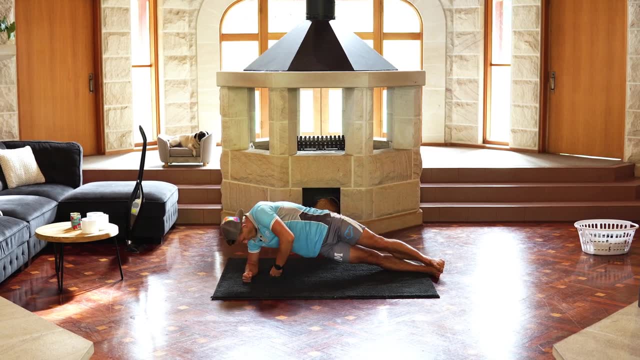 And then I'm going to bring it all the way down Through my body And back up. Okay, Let's go in there again All the way through. It's really tough. You've got to keep going for 30 seconds. 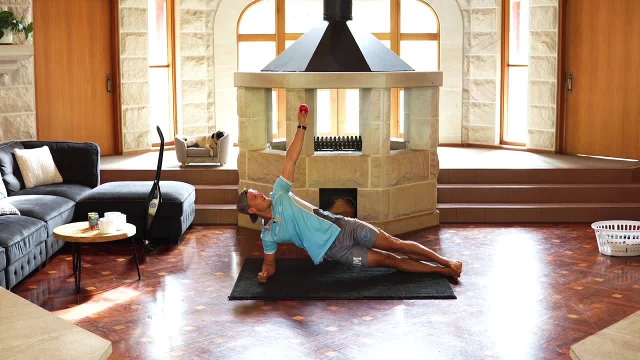 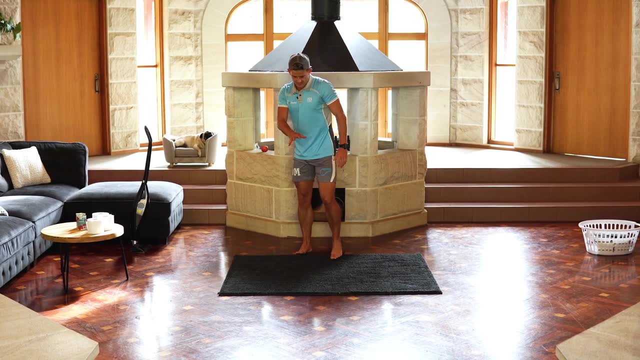 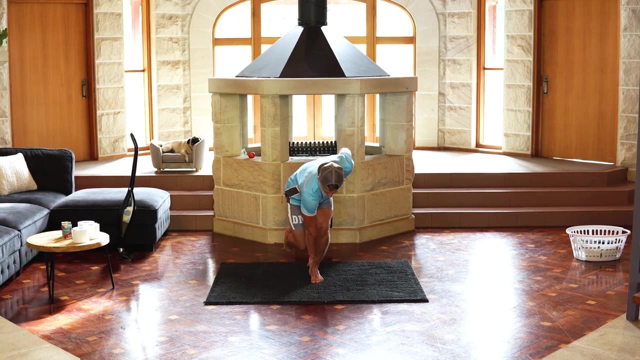 Awesome, There we go. Alright, We've got two more left. On a soft spot again, You've got to balance on one foot And you've got to reach with your opposite hand. Touch your foot Once you touch your foot.